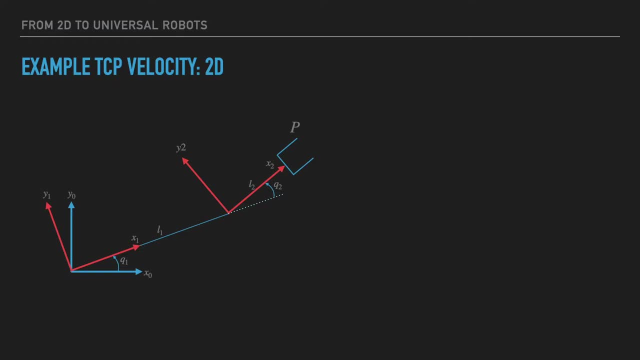 We want to calculate the TCP velocity of point P. For that we need to calculate the transformation matrix of system 1 and system 2.. By multiplying these two matrices we get the transformation matrix of the system Great. In order to get the origin coordinates of point P, we need to multiply the transformation matrix of the system with the matrix of point P. 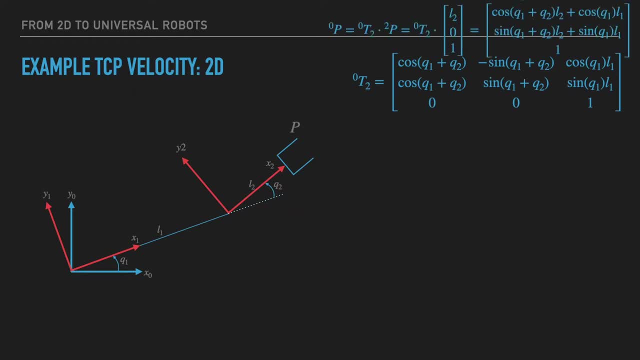 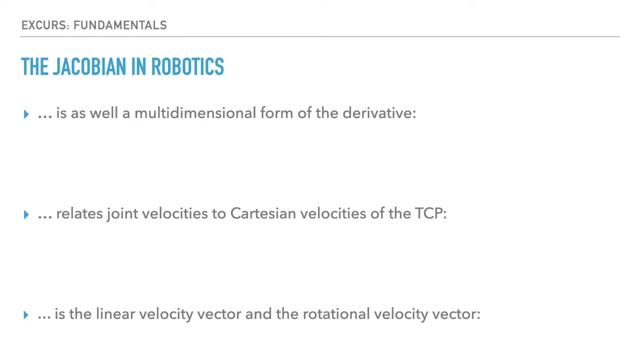 vector of point P in system 2.. The result will be the x and y components of point P in the origin coordinates. The Jacobian matrix in robotics is a multidimensional form of the derivative 2. It relates joint velocities to cartesian velocities of the TCP. 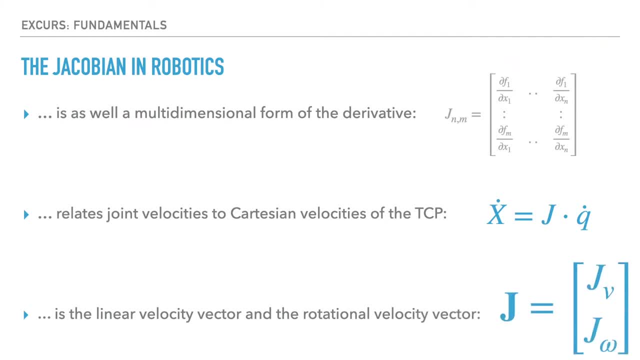 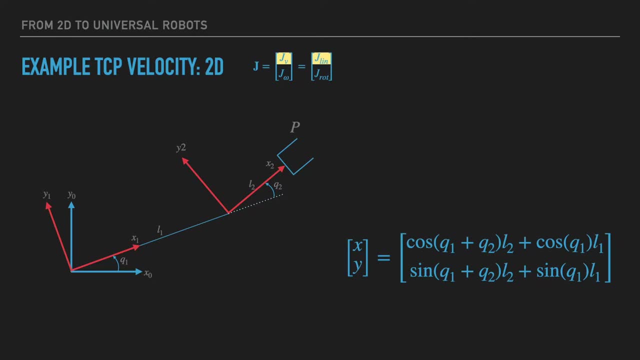 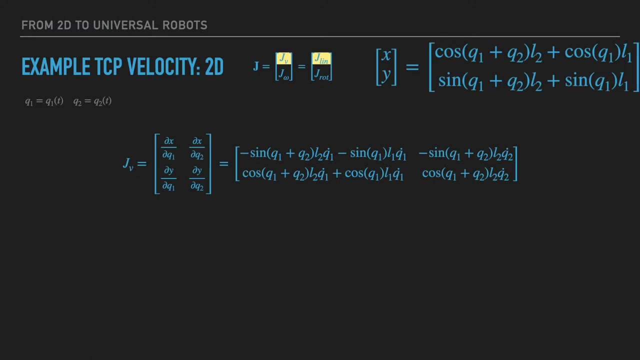 And it's the linear velocity vector and the rotational velocity vector. Let's switch back to our example. We now want to calculate the linear velocity. In order to do that, we need to make the angulas time dependent. We will then form the derivatives. 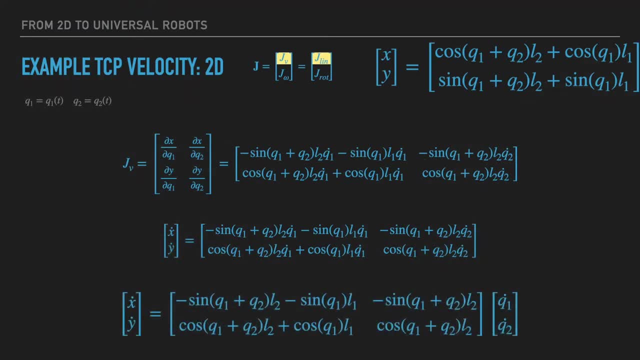 The result will be the x and y components of point P in the origin coordinates. we will then merge the Please, marsians, p and T. The INSANES will be the linear velocity in x and y components of point P in the origin. 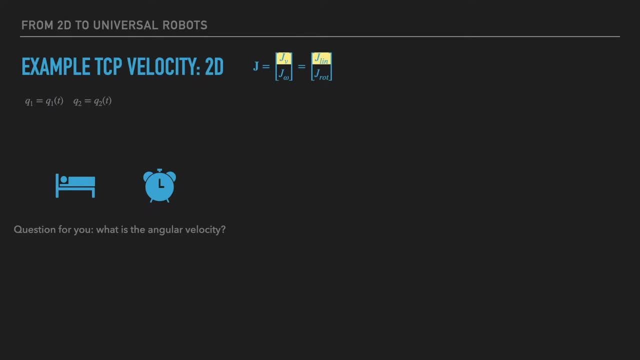 coordinates. Let's calculate the rotational velocity. Before you fell asleep, a question for you. Think about it. pause the video for 1 minute. What is the angular velocity? The angular velocity is nothing more than just H times the physical difference of x3.. 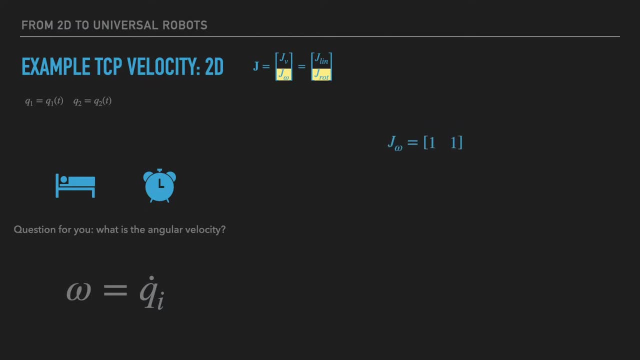 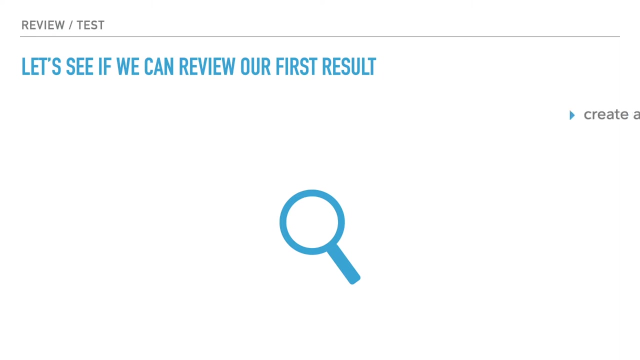 summing up all the velocities, our overall Jacobian matrix will look like this: with this formula we get x and y component of the velocity, as well as the rotational velocity of the TCP. let's see if we can review our first result. we will create an easy example and calculate a TCP velocity with the. 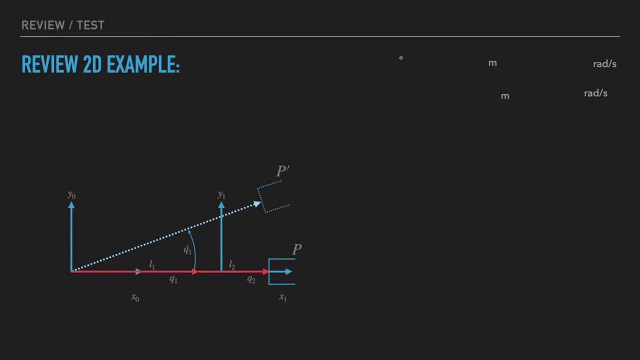 physical model. this is the formula to calculate the TCP velocity. the starting angular of our joints is zero. the length l1 is one meter. the length l2 is one zero point one meters. the rotation is just in y component, which is one point three watts per second. the X rotational 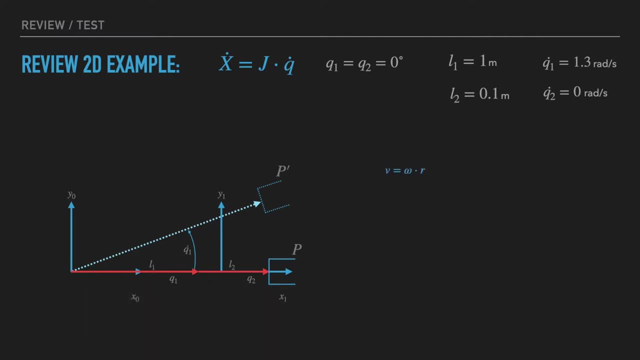 component is zero. in order to get the velocity, we need to multiply the angular velocity with the radius. for our example, it looks like this: we just add up the velocities and the length and our result is one point four three meters per second. let's use our formula to evaluate the Jacobian for the 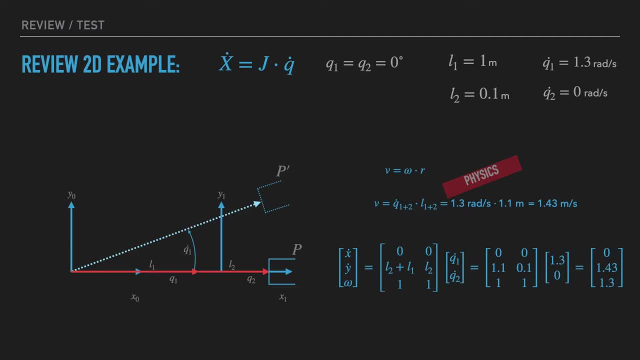 Jacobian, we need to calculate the derivatives. as you can see, the y component of our physical model is the same as we calculated with the Jacobian. you can also see that there is no movement in X component, which means that this drawing is not 100% correct. in reality, the y-axis is showing towards us. 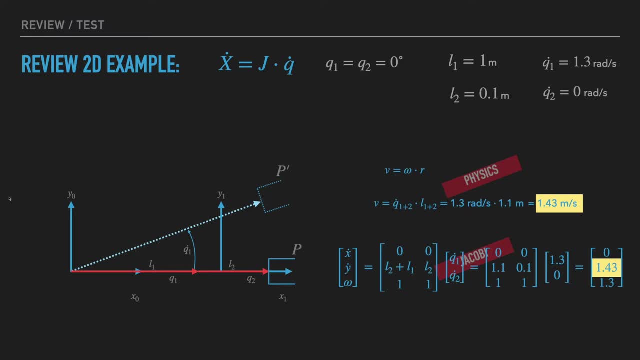 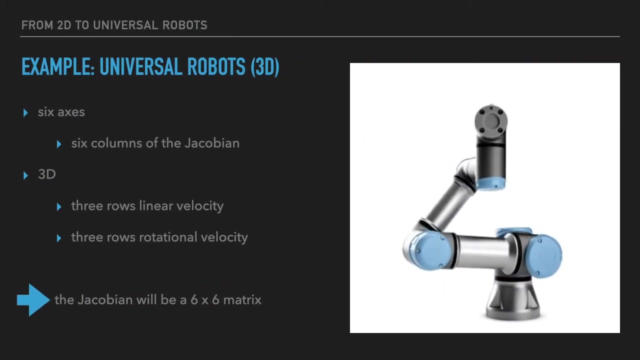 and point P is rotating around it. nevertheless, we can show that the result of the velocities are the same. let's switch to the universal robot example, a 3d example. we have six axis, which results in six columns of the Jacobian. we are in the three-dimensional. 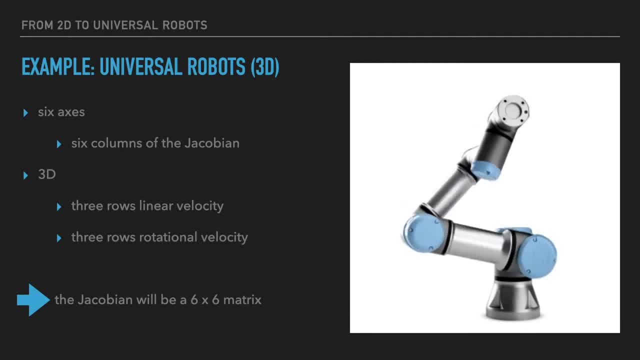 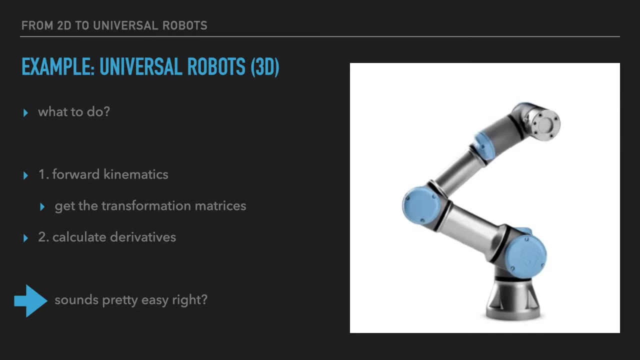 room, which means we have six degrees of freedom, which results in three rows of linear velocity and three rows of rotational velocity. the Jacobian will be a six times six matrix. so what we need to do, we need to get the transformation matrix in order to calculate the forward kinematics. then we can calculate the derivatives sounds. 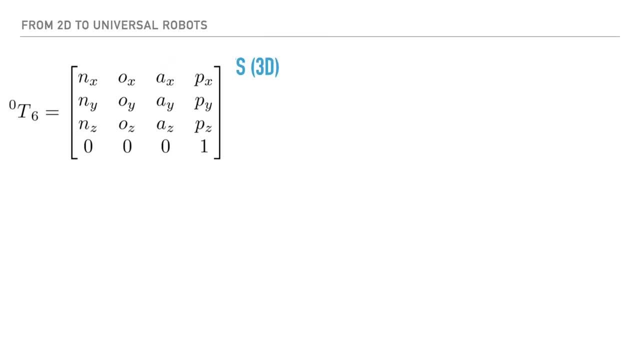 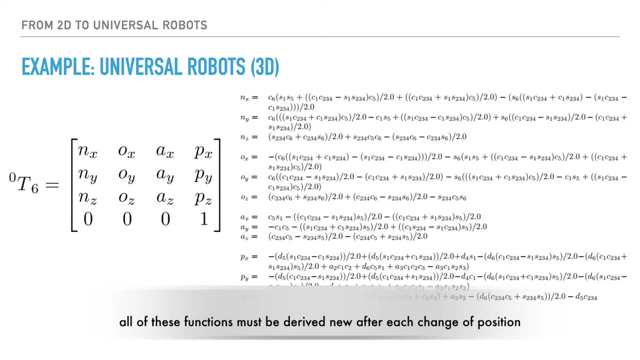 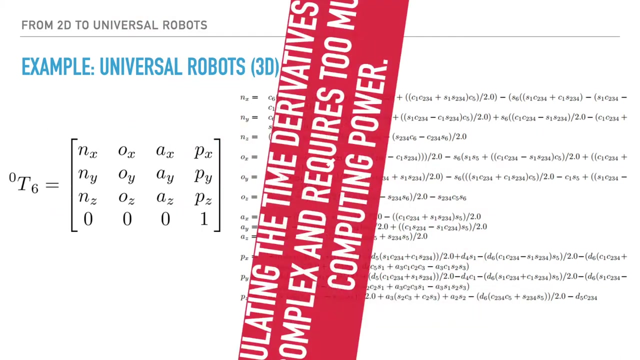 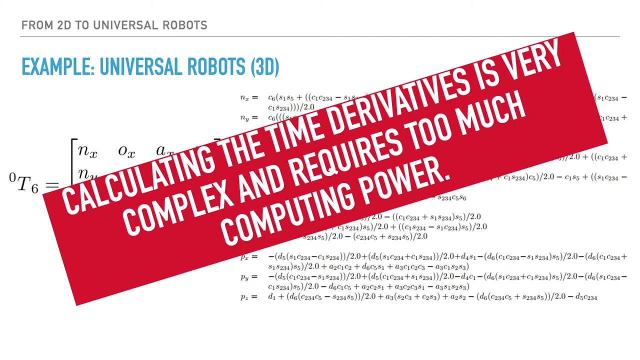 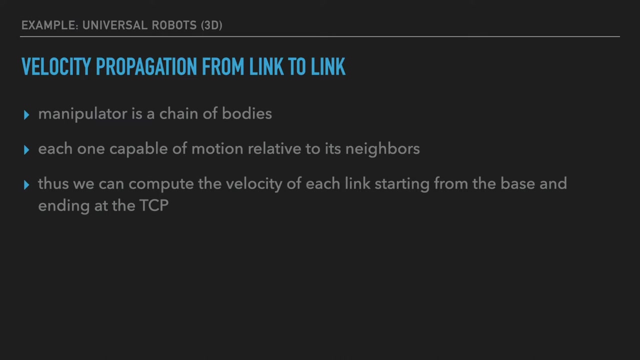 pretty easy, right? this is the transformation matrix and this are all the parameters we need to calculate. it requires too much computing power. luckily, I can show you the velocity propagation from link to link. the manipulator is a chain of bodies, each one capable of motion relative to its 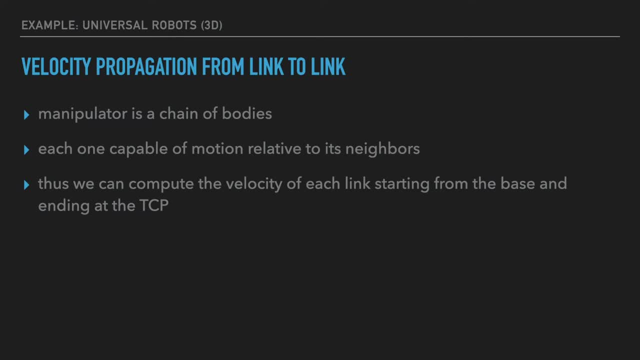 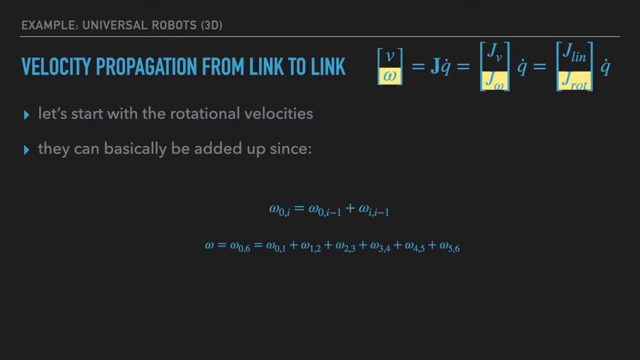 neighbors. plus we can compute the velocity of each link starting from the base and ending at the TCP. let's start with the rotational velocities, since they can basically just add it up. we have six joints, so we add all the six rotational velocities to get the overall rotational velocity, thanks to the 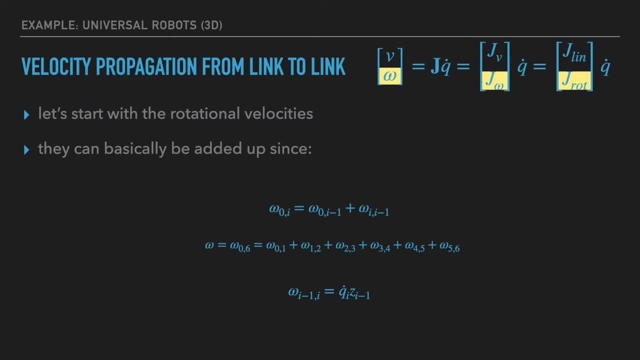 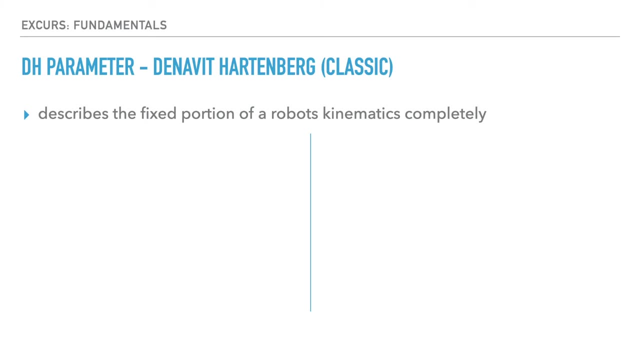 denavid hartenberg parameters. we can use this formula: wait, what are the denavid hartenberg parameters? jack denavid and richard hartenberg introduced this convention in 1955. it describes the fixed portion of a robot's kinematics completely. you can see three joints in this picture. the 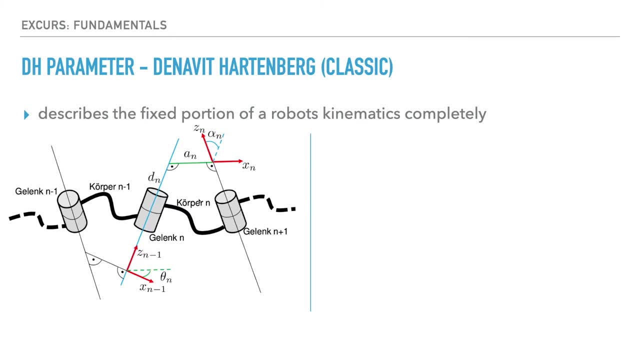 length means joint in German. you can see two bodies. kappa means body in German. we will now draw a straight line which goes through each joint be connected two lines. we are common perpendicular. this results in an offset D which goes from here to here in an angle. theta of old X and new X, a length of common normal a and an angle. 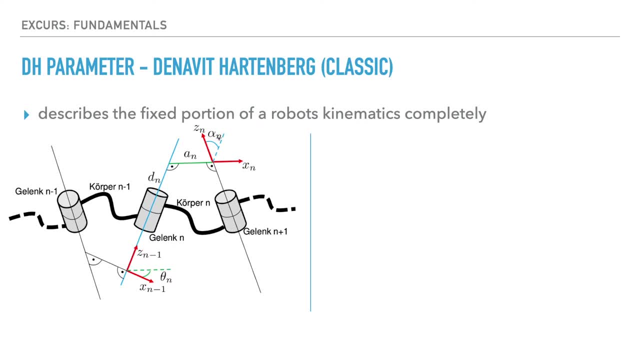 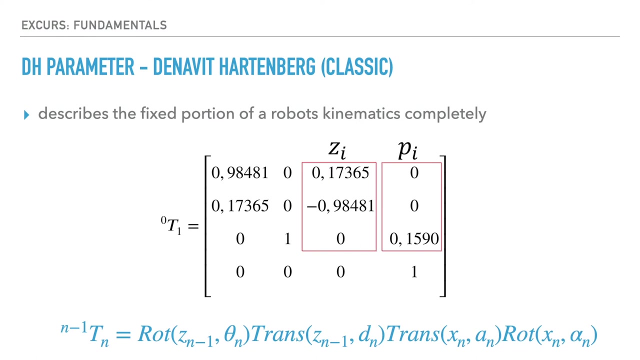 about common normal alpha. the denavid hartenberg parameters for universal robot looks like this: you. with the help of this convention, the transformation matrices of a system can be determined via the following relationship: our set is stored in the transformation matrices. pause the video now and do a research on the modified DH. 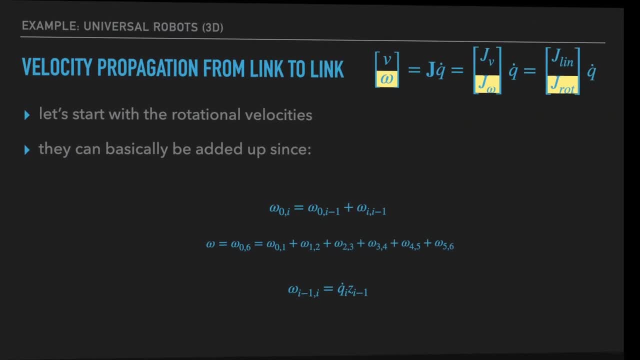 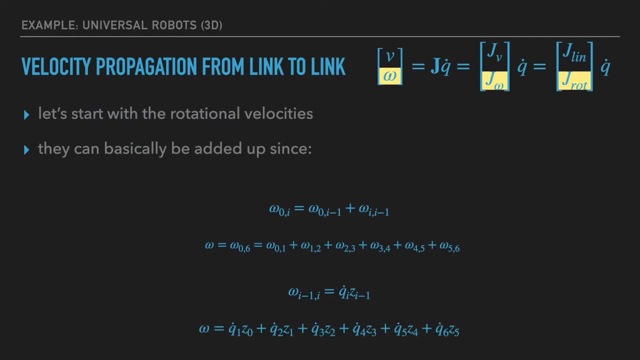 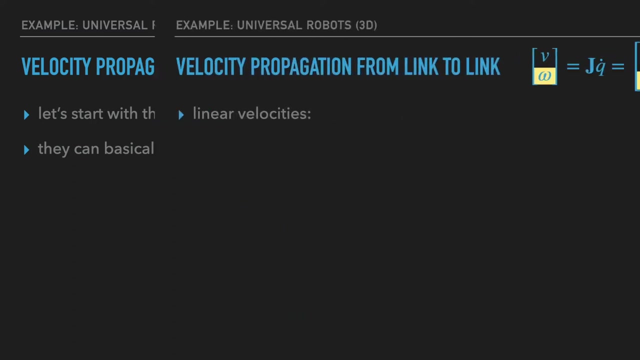 parameters back to the velocity propagation from link to link. we can add up all the rotational velocities with the set components. this results in the rotational portion of our Jacobian matrix. great, and now the linear velocities from the physics. we have this formula in the three-dimensional room. it 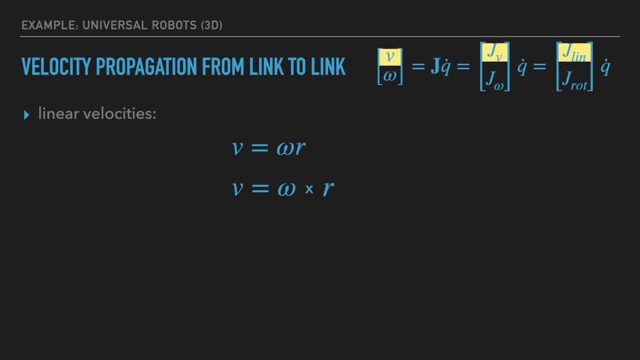 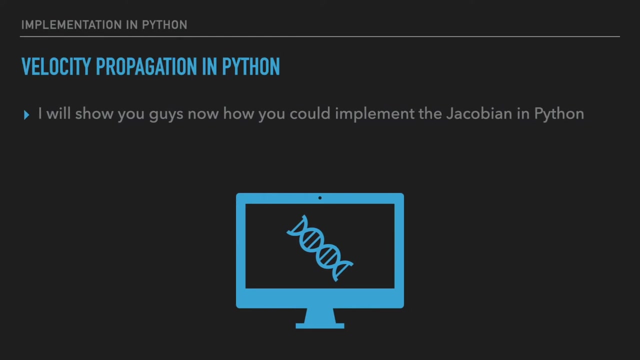 means to form the cross-product between Omega and R, and this means nothing more than adding up the previous velocity to the current velocity. the formula gets more clear in the Python program. let's switch to Python. I will now show you guys how you could implement the Jacobean and Python, the. 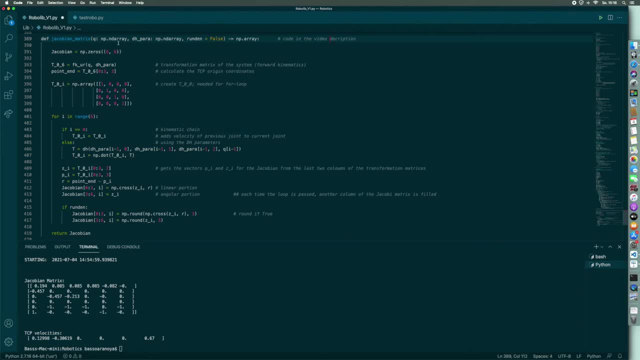 formula gets more clear in the Python program, let's switch to Python. I will now show you guys how you could implement the Jacobian and Python. Here you see the function: Jacobian matrix. By the way, the code will be in the video description. First we will create an empty matrix. 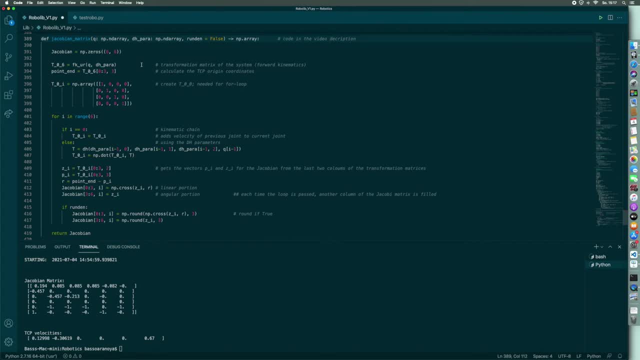 Then we will calculate the transformation matrix of the system. with the forward kinematics to calculate the TCP origin coordinates, We will create the transformation matrix of system 0 which is needed for the for loop. The for loop starts here. This is the actual kinematic chain. 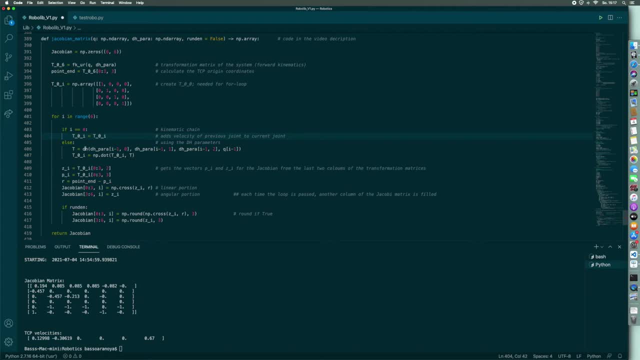 It adds the velocity of the previous joint to the current joint using the dh parameters. The results are stored in the transformation matrices. Down below here we get the vectors p and z for the Jacobian from the last two columns of the transformation matrix. Down below here we get the vectors p and z for the Jacobian from the last two columns of the transformation matrix. 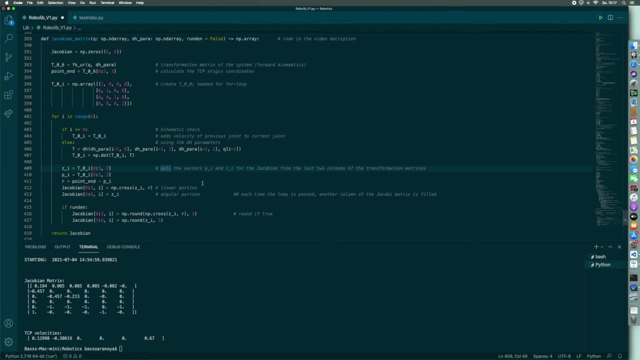 Down below here we get the vectors p and z for the Jacobian. from the last two columns of the transformation matrix We get the linear portion and the angular portion down below here. Each time the loop is passed, another column in the Jacobian matrix is filled. 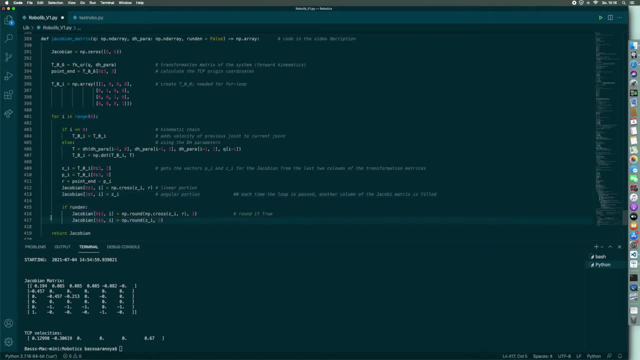 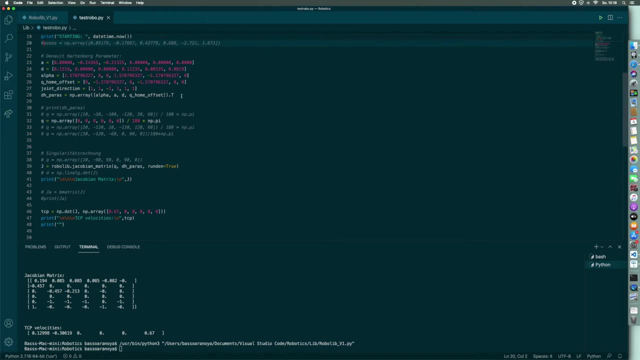 Down below. here we just round our results. Let's run the code. We switch to our test script. Here you see the Dynavid-Hartenberg parameter stored in the dh parameters. Here you see the Dynavid-Hartenberg parameter stored in the dynavid-Hartenberg parameter. stored in the dynavid-Hartenberg parameter. 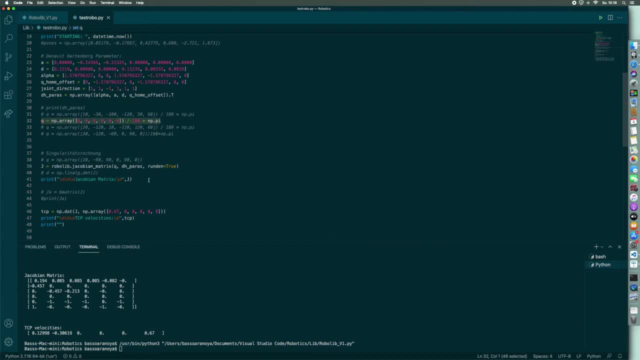 These are the start angulars from all the joints Down below. here we calculate the Jacobian and print it. Here we calculate the tcp velocity and print it. Let's run the code. You can see the Jacobian matrix here, as well as the tcp velocity here. 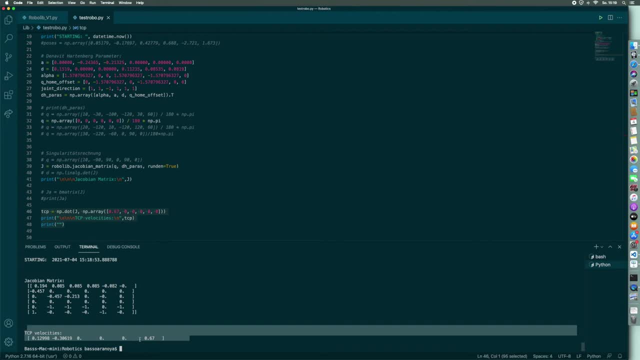 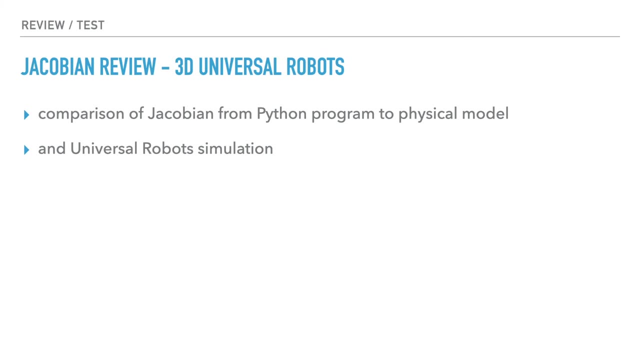 You can see the Jacobian matrix here, as well as the tcp velocity here. Remember this and we switch back to the presentation. the presentation. Let's review our results from Python. We will compare the Jacobian from the Python program to the physical model as well as to the. 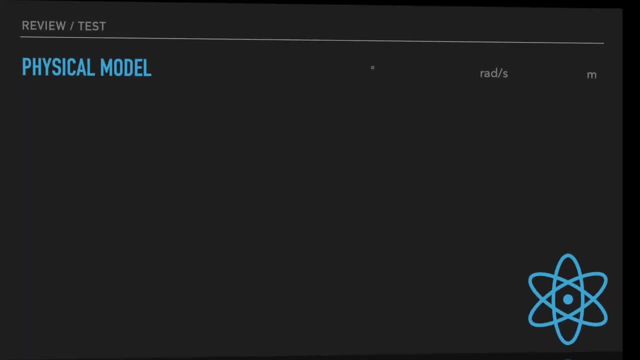 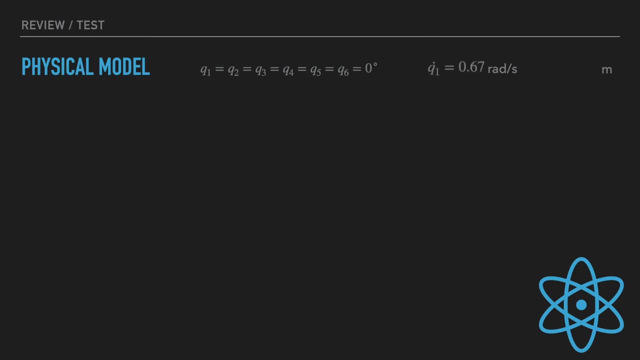 universal robot simulation. Let's start with the physical model. Our start angulas are zero degrees, We only have one movement of 0.67 watts per second and the length is 0.46 meters. Our velocity is calculated and the result is: 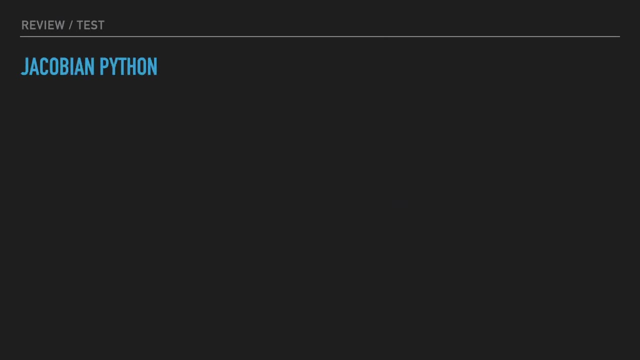 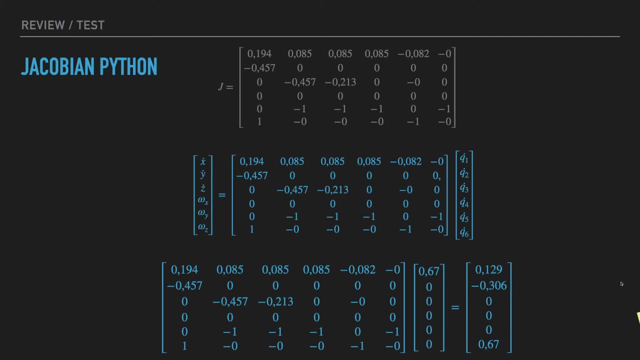 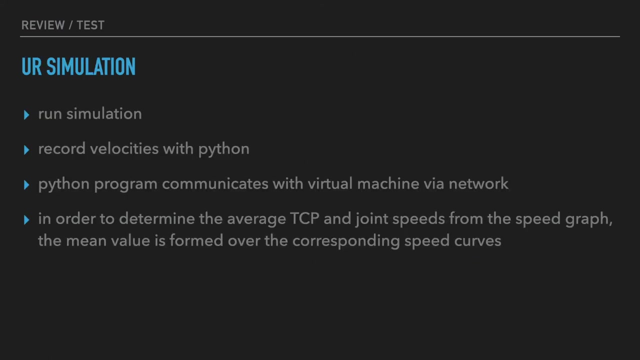 0.31 meter per second. The Jacobian from Python, You remember the Jacobian. In order to calculate the TCP velocity, we take our formula and result in this vector. As you can see, the result is pretty similar to our physical model. Let's start the UI simulation. I run the simulation, record the velocities. 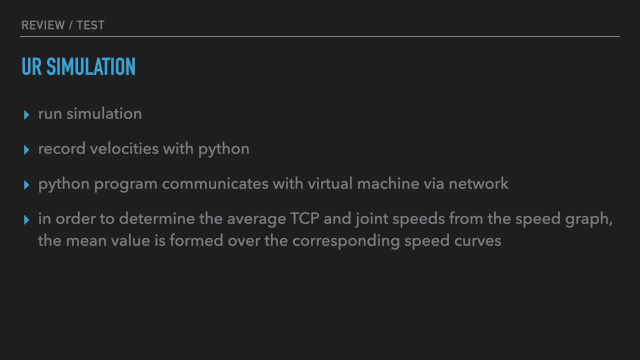 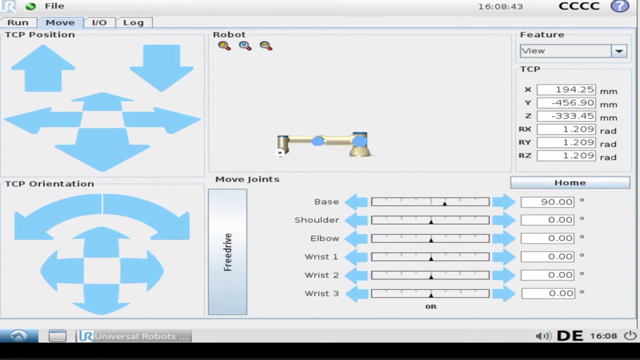 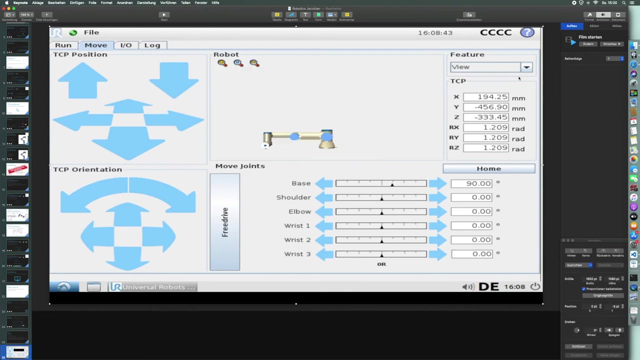 with Python. The Python program communicates with the virtual machine via network. In order to determine the average TCP and joint speeds from the speed graph. the mean value is formed over the corresponding speed curves. I recorded the simulation. You can see the simple movement. The simulation will: 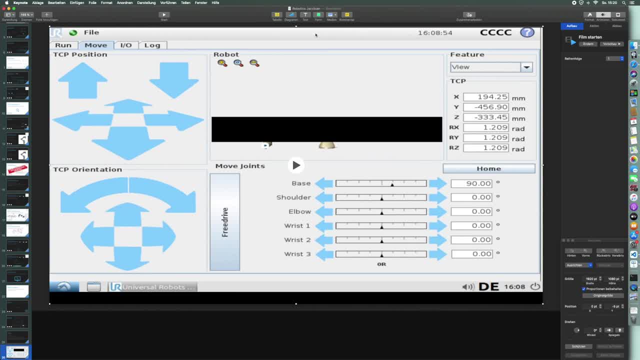 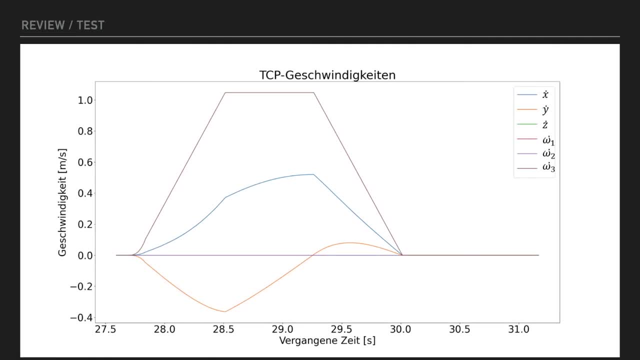 send all the velocities and other parameters to the Python program. The Python program creates this graph. Here you can see all the TCP velocities: X, Y, Z and Omega components. If you calculate the mean value, you will have the same result as our Python.